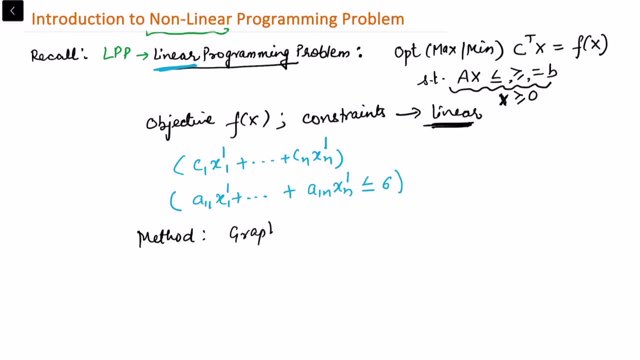 methods such as graphical. and then we have done various simplex method and its variance. When I say simplex method, which means we are including big M, two phase revised simplex method. So simplex method and its variance can solve the linear programming problem. We have also learned using 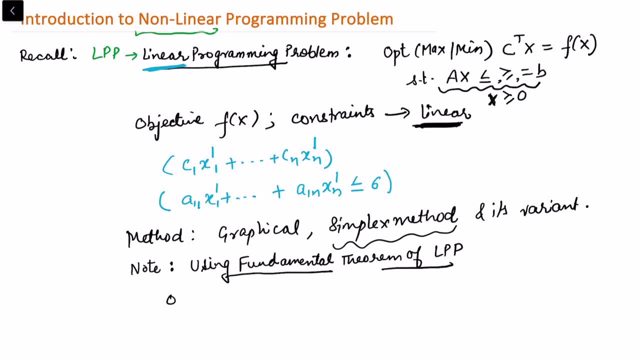 the fundamental theorem of linear programming problem that the optimal solution In the linear programming problem this lies at one of the extreme point. This lies at one of the extreme point and generally these extreme points are the corner point, which we also call this as basic feasible solution. And of course the region has to be provided. the region is convex polyhedron. 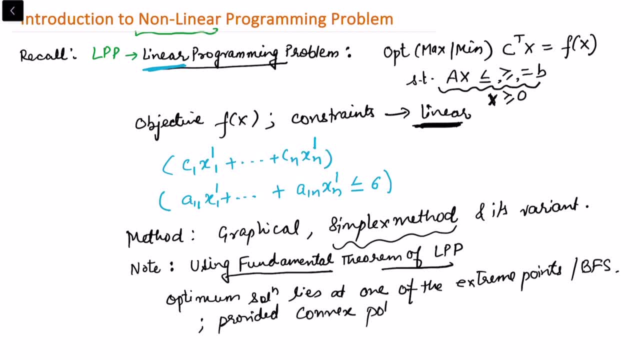 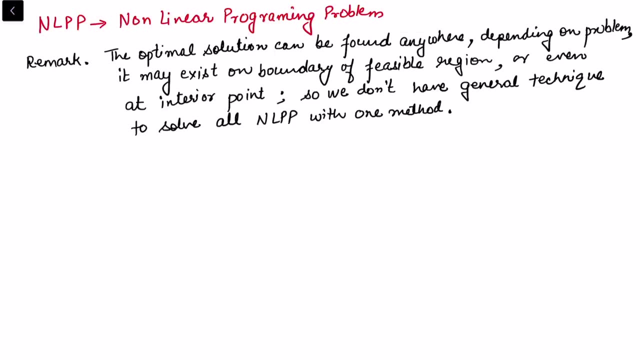 So the region convex. polyhedron means it is a bounded and without any holes polyhedron feasible region. So this is the restriction on the All these topics method and these details I have covered in my last videos. link added in description. But in case of nonlinear programming problem the optimal solution can be found anywhere. 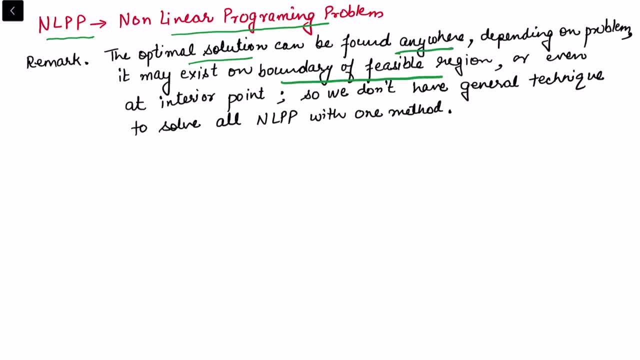 depending upon the problem, It may exist on the boundary of the feasible region, or even it may exist in the interior point. Now, this was not the case in the linear programming problem. We do not find the solution in the interior point, If at all. the solution lies in the interior point that 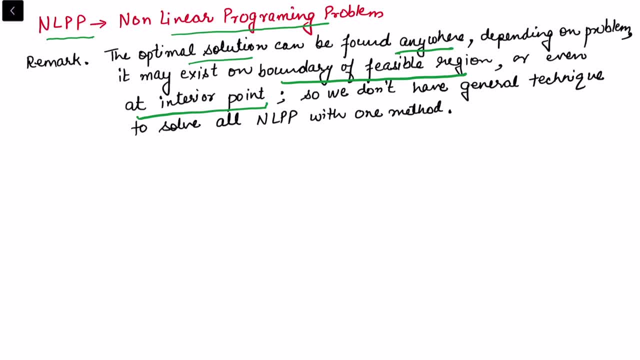 means the function was constant. So in this case we have to find the solution in the interior point. The nonlinear programming problem. we may even have the solution at the interior point. So we can say we don't have a general technique to solve all nonlinear programming problem with one method, So we have to. 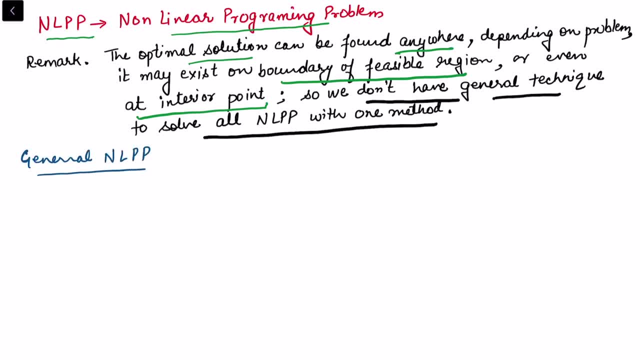 make different categories. So let's first consider the general nonlinear programming problem. So there again we have some function which want to optimize subject to certain constraint and constraint. I'm showing it by g, i, x, less than, again greater than, or the constraint may be equal. There may be some. 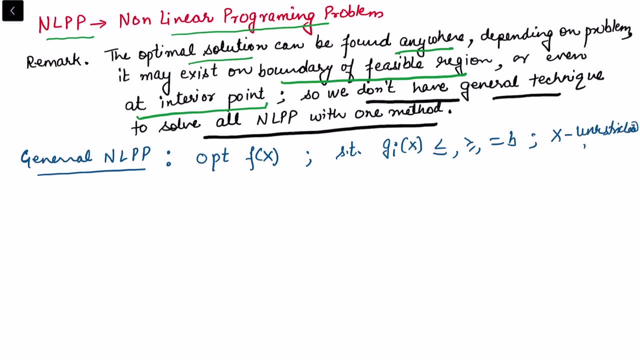 restriction on the decision variable, or they may be unrestricted. So I'm just adding both. So this is same structure. We have an objective function, Then we have some constraint and then we have the restriction on non restriction on the decision variable value. Now, if f of x or g i x or both are nonlinear, So that 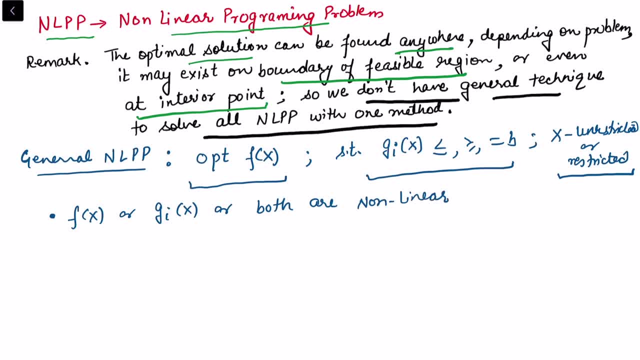 means if either the objective function is nonlinear, then we say it is a nonlinear programming problem, The constraint a nonlinear, or both of them are nonlinear, Then we will say that this is a non linear programming problem. for linear programming problem, everything has to be linear, But for nonlinear, if anything, 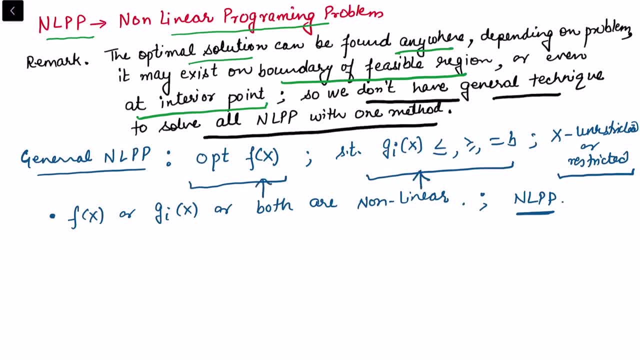 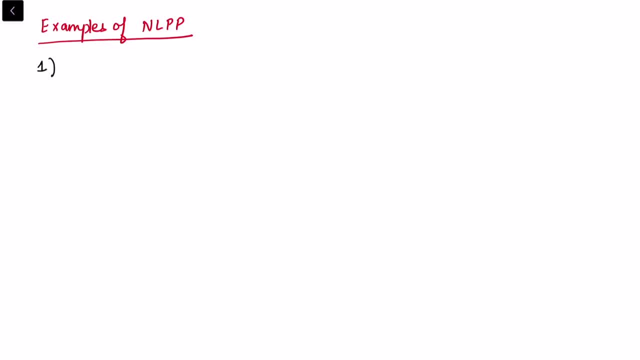 either the objective function or any of the constraint is nonlinear. we will put this into the category of nonlinear programming problem. So now we take some examples for the nonlinear programming problem. Suppose I want to find the maximum of f of x equal to x, 1 square plus x. 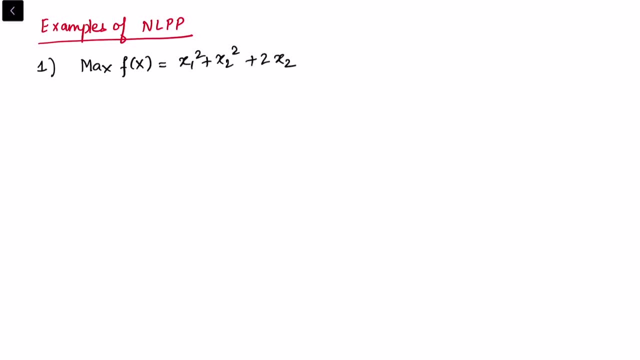 square plus 2x2. you see that this is simply an objective function and there are no constraint, and these problem are something that we usually solve with the help of the calculus techniques. so, for example, let's take another very simple here. i take y square equal to x, or i can simply: 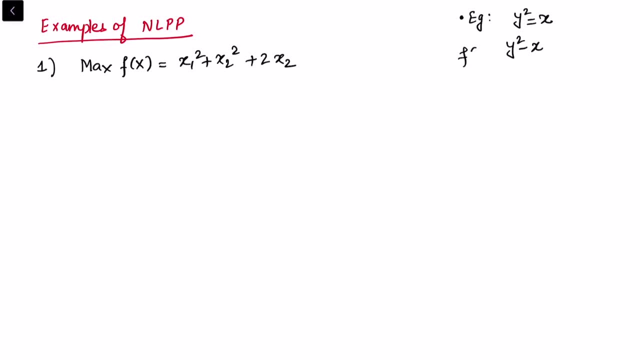 write that this is a y square minus x, and let's call this as function capital f of x. or you can even rename that capital f of x equal to x2 square minus x1. so x2 is my y and x1 is x. in this case you can have, let's say, x1 is here and x2 is here, and this is the shape of the parabola. 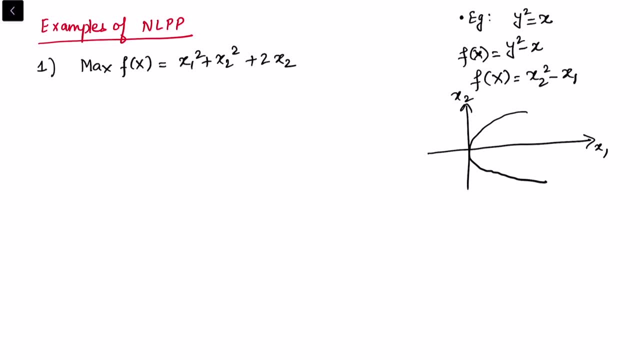 and we want to find the maxima or the minimum value. it may exist or it may not exist, so it depends upon. we'll be using the techniques based on the calculus. so this is the first type of the non-linear programming problem, which is without constraint, so we can say: 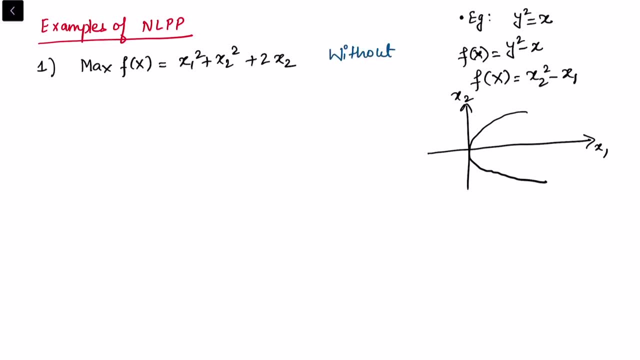 you, There are problems in the non-linear programming problem which are without constraints. Then there are some examples where we can have the constraint as well. Say, I want to find again maximum of f of x, which is x1 square plus x2 square, But this time there are some constraint: x1 plus x2 greater than or equal to 4.. 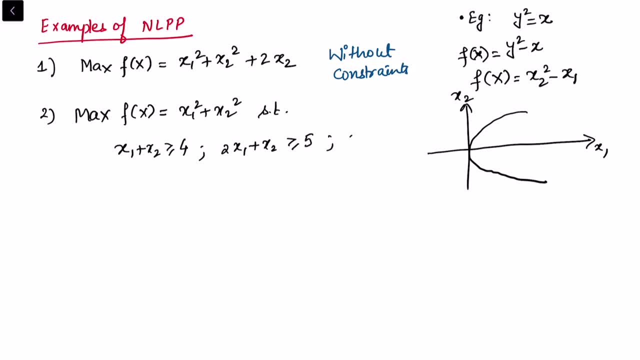 2x1 plus x2 greater than equal to 5, and even there are some non-negative restrictions. So here I have taken constraint with inequality. So it says with constraints, and the constraints are also with inequality. So we can say: with inequality, constraints. 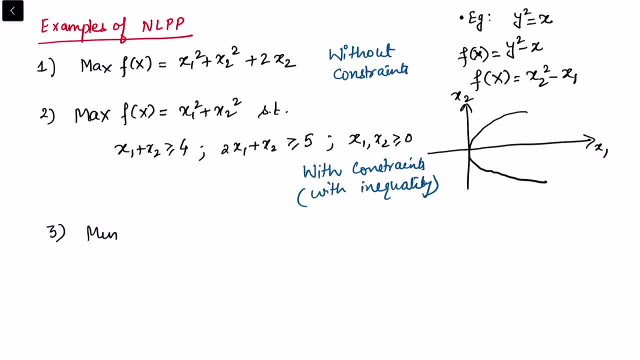 Then there are some problems where we can have- let's say you take another example- f of x, which is equal to 2x1 square minus 24x1 plus 2x2 square Minus 24x2 square, Minus 24x2 square. 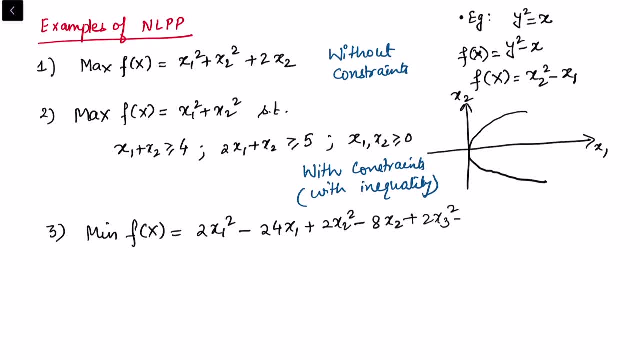 Minus 8x2 plus 2x3, square minus 12x3 plus 200, subject to some constraint with equality sign. So now I am taking a constraint where the constraint is equality and then you have some non-negative restriction. So this we will put with a constraint, but the constraint is with the equality sign. 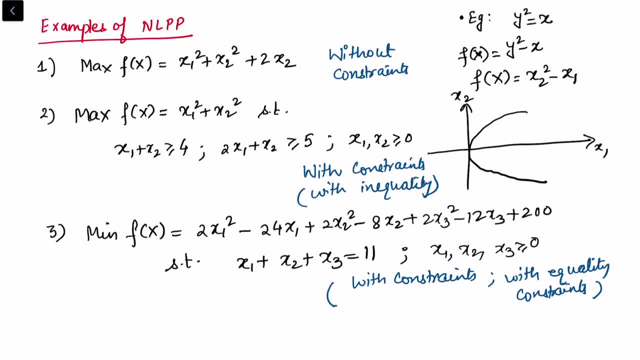 So we can say: with equality constraint, So we have this as another type of the problem. We can see that again: This is without constraint, So there are no constraint. There are certain constraint with inequality. So you can see: constraint have inequality sign. 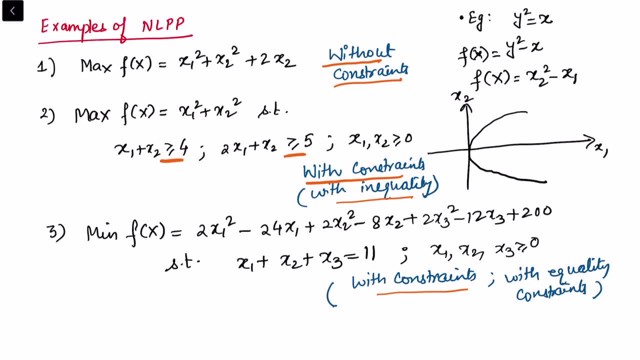 It is not equality and then there are certain constraints with the equality sign. You can see that. then there is another format. Say you consider specifically quadratic form? quadratic forms are something where the objective function have, So this is again without constraint. I'll add here: 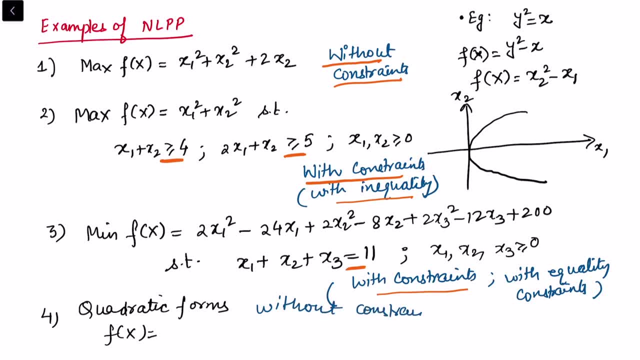 This is also without constraint, And in this constraint each term appear with the degree 2.. So for example, we can say x1 square plus x2, square plus 5 times x1, x2.. Now you notice, here the total degree of each term has to be 2 always. 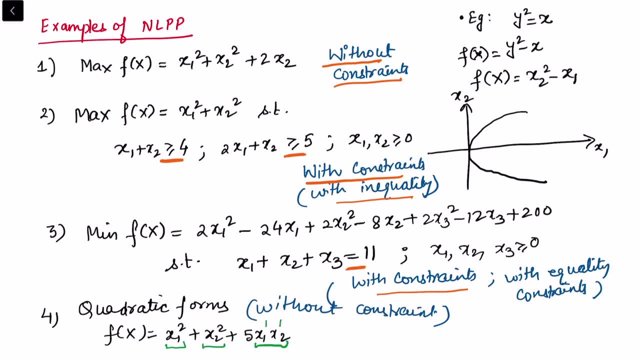 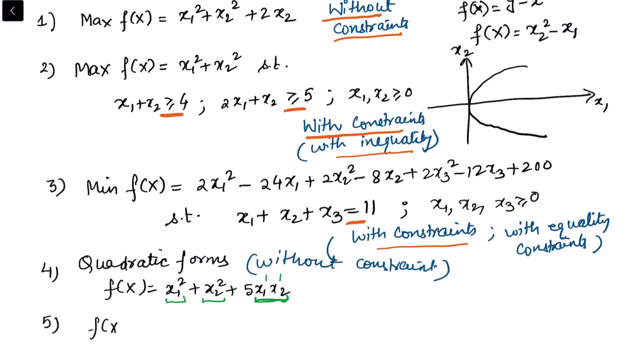 So x1 is also coming with degree 1 and x2 is also coming with degree 1.. So the total degree of this term is 2.. If I take another example, something like this: f of x, which is equal to x1 square plus x2.. 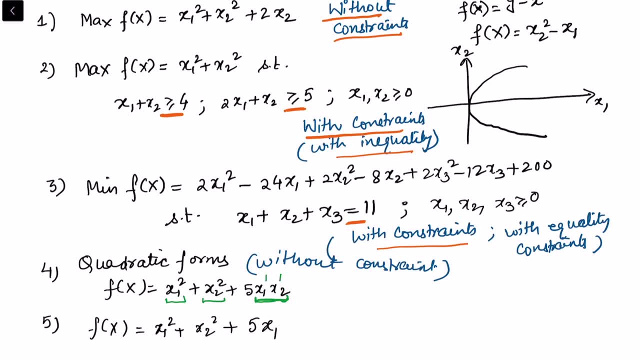 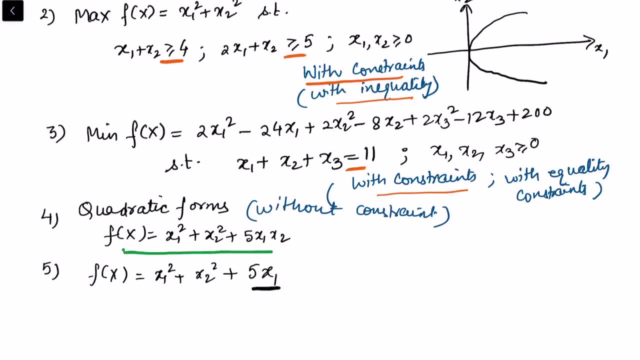 x2 square plus 5 times x1.. Now this is not called as quadratic, because here this term have degree only 1. So we can see that if the function have a quadratic form or a non-quadratic form, that further become a category in the questions without constraint. 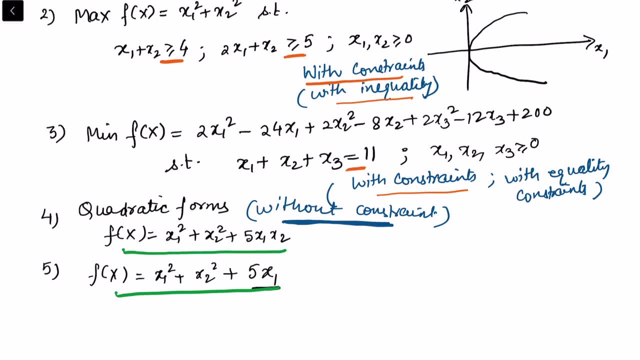 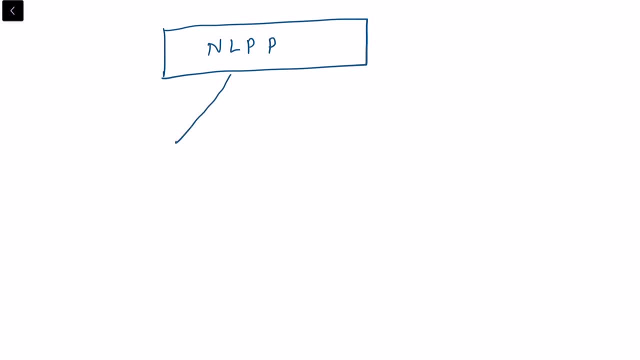 And we'll be learning the concept of Hessian matrix or bordered Hessian matrix. So now we can finally say that let's consider a non-linear programming problem. It has two categories. Let's first broadly divide- This is without constraint, and on the other side, I will consider this with constraint. 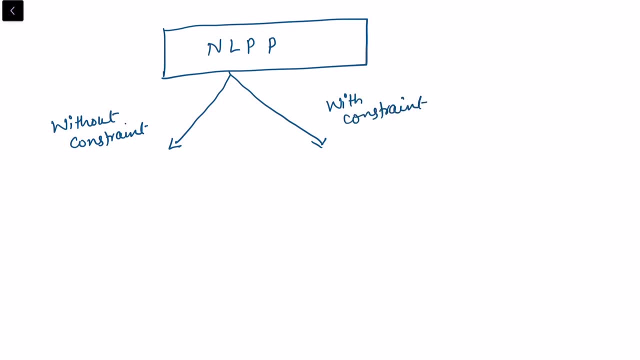 So, depending upon which problem it is, we'll apply the method Without constraint. again, we will look whether the problem is quadratic form or not. Quadratic form, I've just explained. Each term in the degree has to be 2. The total degree, or if it is non-quadratic form, 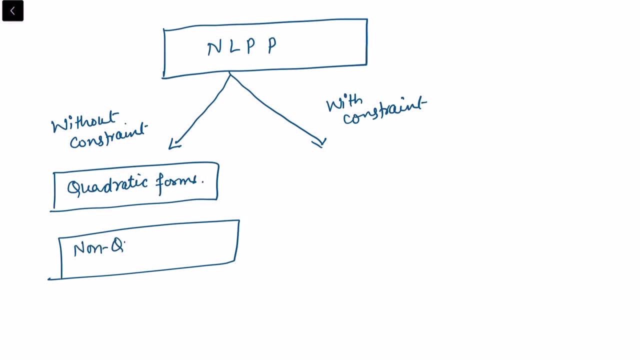 So another possibility here is non-quadratic. So either we can consider quadratic form or we can consider non-quadratic form. For this we will construct Hessian matrix, and for this Hessian matrix reduces simply to symmetric matrix. Now here with constraint, if the constraints are inequality constraint. 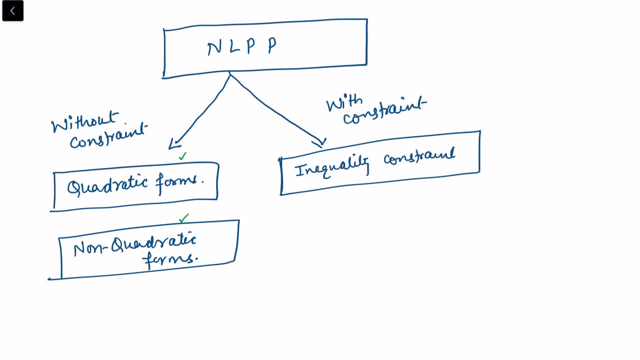 So, if I consider inequality constraint, So in this case we will apply the method which we call it as KKT conditions or KKT criterias. Now, these are necessary and sufficient conditions. So if the both conditions- necessary and sufficient condition- will verify and we will substitute that. 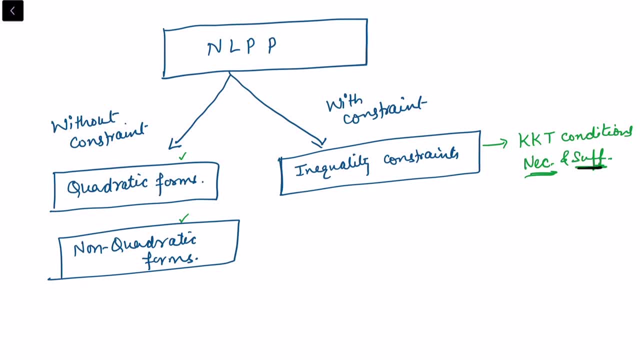 So the moment we say it is sufficient condition, will just have to verify those sufficient conditions are satisfied. We'll talk about maxima or minima. Similarly, if the constraint are with equality constraint, So then we will apply here the method which we call Lagrange multiplier. 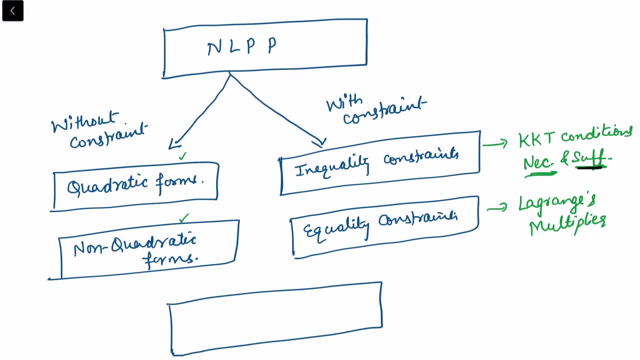 So here we'll apply Lagrange multiplier. So here we'll apply Lagrange multiplier. Apart from these, there are certain search technique methods also. Suppose these methods are not working and we'll apply the numerical analysis techniques or techniques by trial and optimize. So these are called search technique methods. 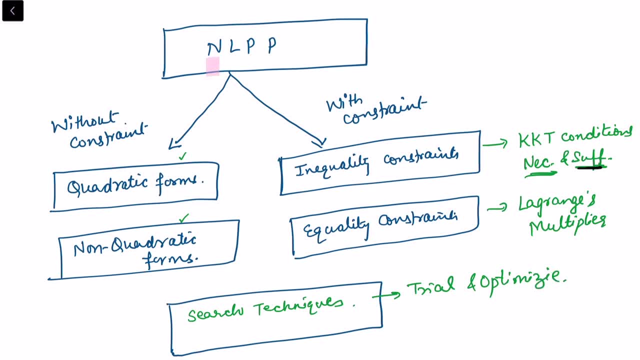 And in the search technique method also, we can look for the solution of a non-linear programming problem. So I'll be covering all these problems in my next video, one by one, And we'll be starting with the without constraint, followed by the problems with the constraint, with the method. 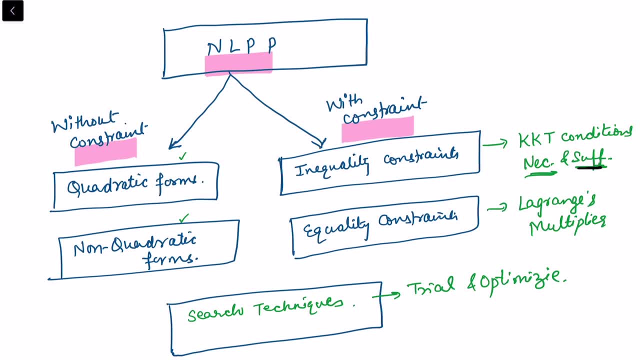 That I've just explained. So we'll see you in the next video. Bye, bye discussed, but before i end this video, let me to take an example for the formulation of a non-linear programming problem. just to give you a glimpse that we do have a formulation similar to what: 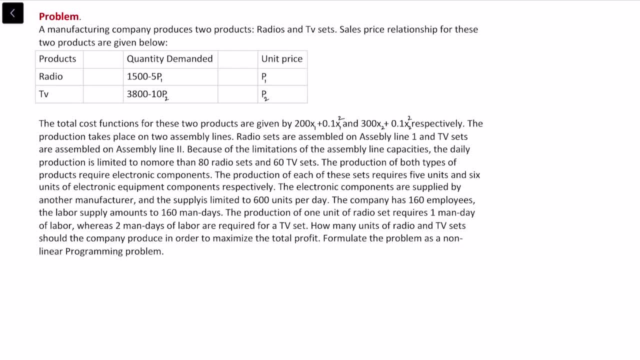 we have done the formulation in the linear programming problem. so we look at this problem and we will formulate this non-linear programming problem. now let's read the problem. a manufacturer company produces two products- radios and tv set- and the sale price relationship for these two products are given in this table. so there are products and then we have quantity demanded and 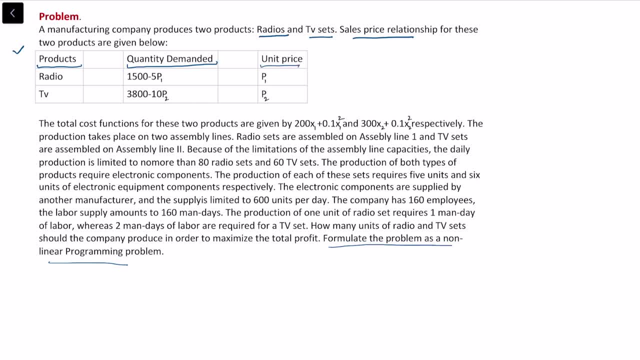 we also have the unit price. the total cost function for the two products are given as this. so this is the cost function, and then we have certain constraint here. so we start our problem with this assumption that whatever is produced is sold in the market. so let's now take the decision. 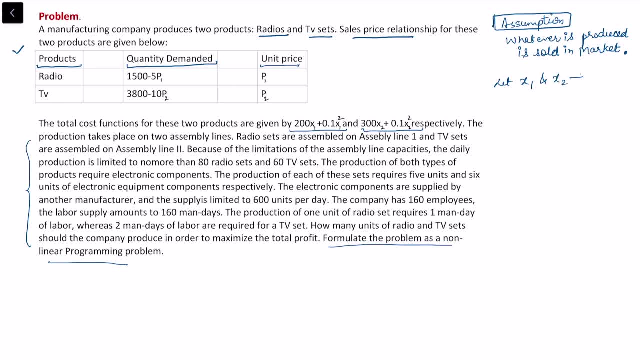 variable x1 and x2. this stands for the quantities of radios and for the tv sets. so quantities of radio sets and tv sets respectively. so these are the two initial restrictions that i have decided for the variable and also done the assumption. it is already given that if we have these quantity as demanded, that means if we are producing this. 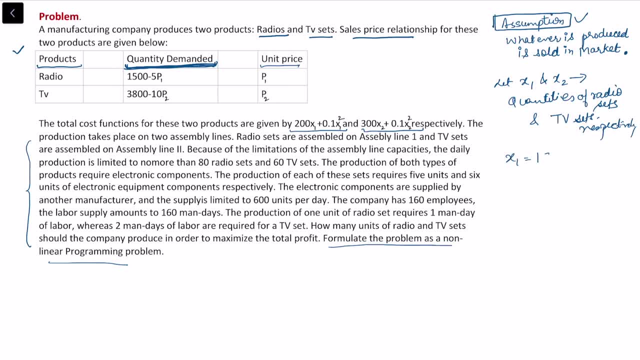 much. so i'll just take x1 is 1500 minus 5 times p1. p1 is the unit price, as we can see here, and x2. this is equal to 3800 minus 10 times p2. from here you can also calculate the. 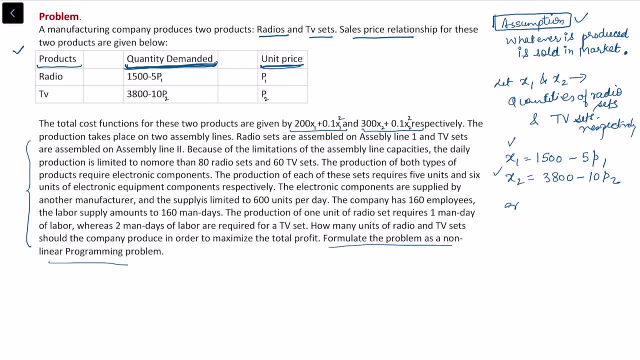 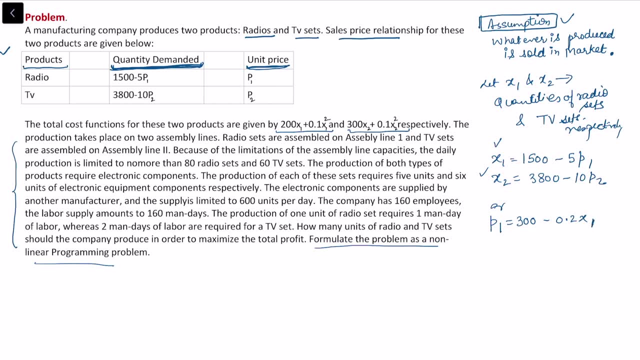 unit price in terms of the quantity produced. so we can simply say: p1 is 300 minus 0.2 times x1. so taking constant on other side we get p1 and p2, which is 380 minus 0.1 times x2. and now let's say: 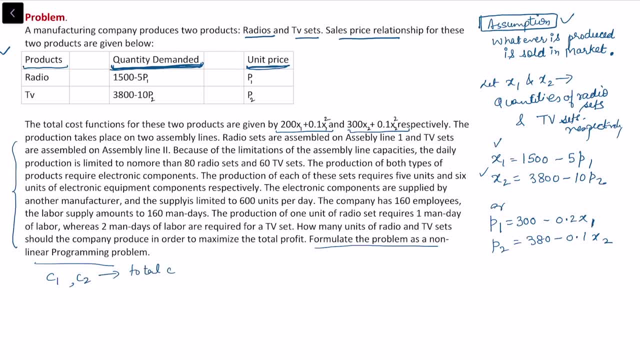 p2. this stands for total cost of production, total cost of production of these units of radio sets and tv sets respectively. radio sets and tv sets respectively. we've been also given that the total cost function of these two product are these. so this is already given to us. we just 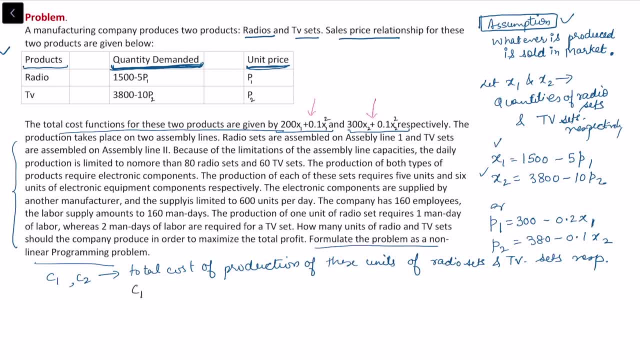 have to pick the cost from the given data. so c1 is 200 times x1 plus 0.1 times x1 square, and c2: this is equal to 300 x2 plus 0.1 times x2 square. so from here we can simply say what is the total revenue. revenue is per unit cost: p1. 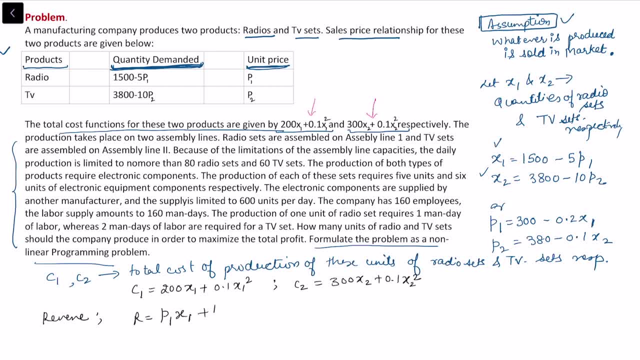 into the number of unit that we desire to produce, plus p2 into x2. so this is per unit cost of radio and the number of radius. or you can say the quantity of the radius produced. p2 is the per unit cost of tv and x2 is the quantity of tv. so from here you can simply say: substitute the value for 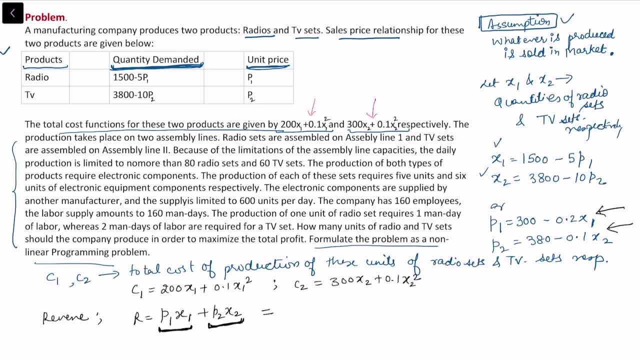 p1 from here and substitute the value for p2 from here. so we get here 300 minus 0.2 times x1 into x1, plus the value for p2, that is 380 minus 0.1 into x2, and then we have one more x2, so we 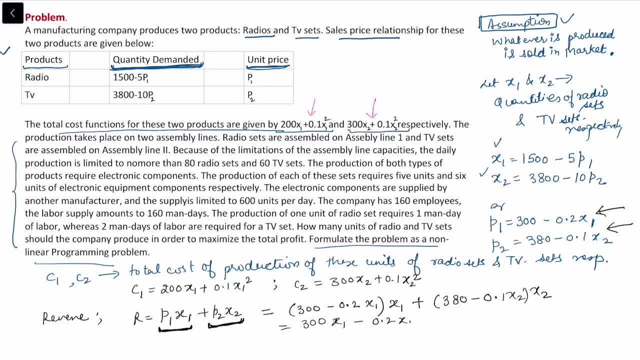 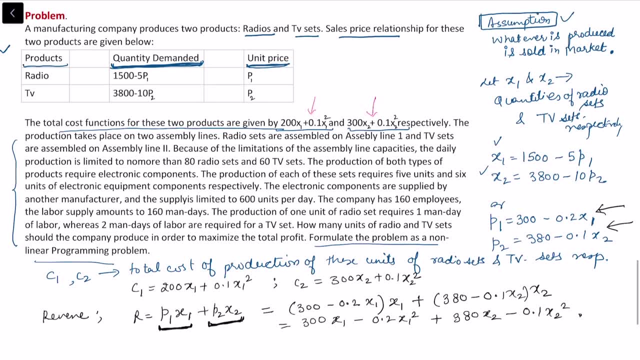 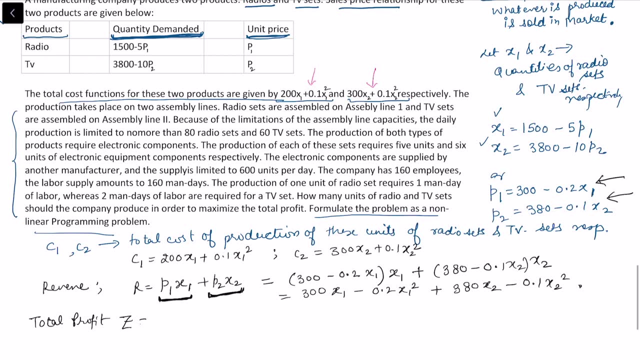 get 300 into x1 minus 0.2 times x1 square, plus 380 into x2, minus 0.1 into x2 square. so the total profit is total profit, which is revenue, and let's say i denote total profit by z, so that is revenue. 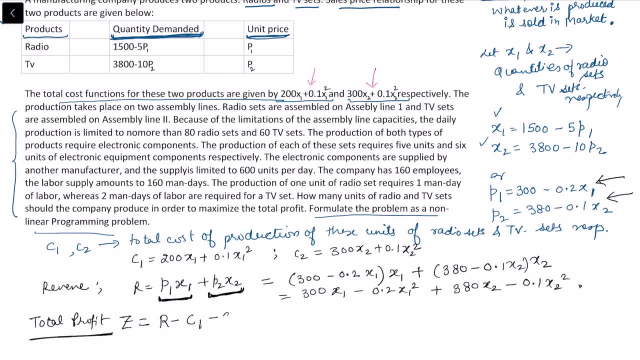 minus the cost expenditure, so that is c1 minus c2, so the cost will be subtracted from the revenue, or we can call this as at this moment, revenue as a sale price, and then we subtract the cost, so that we have already calculated. so now this is the 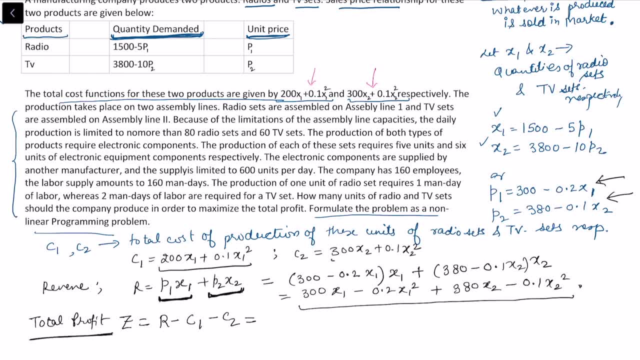 value for r and c1, c2. we have already calculated or we have simply written from the data. so this becomes 100 x1 minus 0.3 times x1 square, plus 80 times x2 minus 0.2 times x2 square. so you notice. 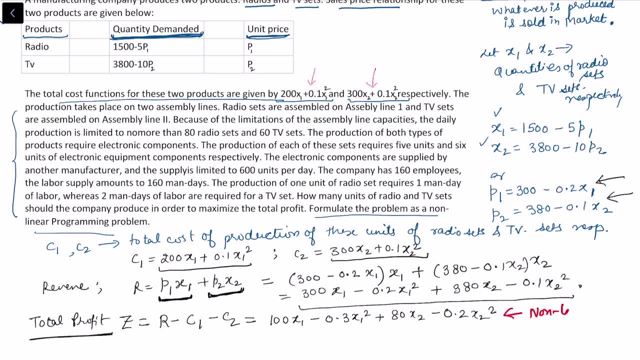 that this is becoming a non-linear function because of the data, how it is given to us, and then we get the objective function as a non-linear. so certainly this is a non-linear programming problem. now we just have to look at the constraint as well. so we have to read what is. 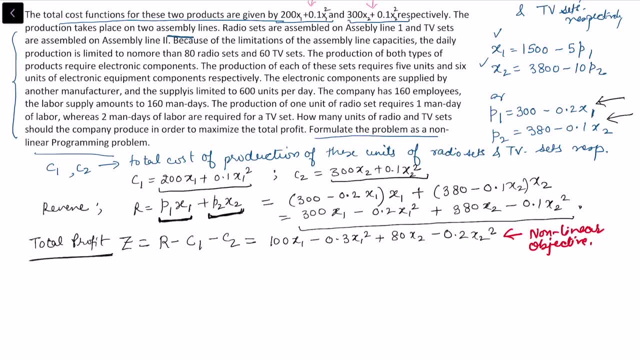 the data given to us, the production takes place on as two assembly lines: radio setter assembling assembled on assembly line one and tv sets are assembled on assembly line two. because of the limitation of the assembly line capacity, the daily production is limited no more than 80 and 60 tv sets. so this means this is the restriction on the decision variable. so we can. 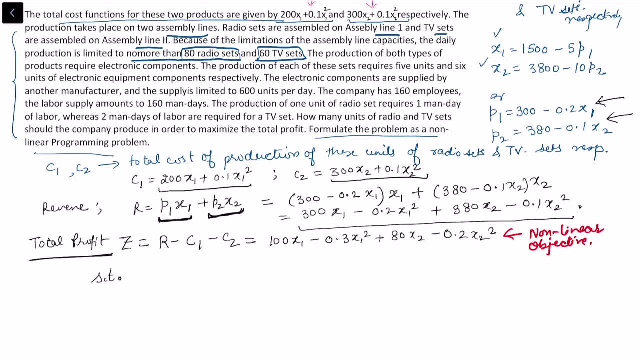 keep subject to the condition that x1 is less than or equal to 80 and x2 is less than or equal to 60. so you can see that this is the condition on the tv set and this is the condition on the radio set. moving forward, the production of these two types of the product require electronic component. the 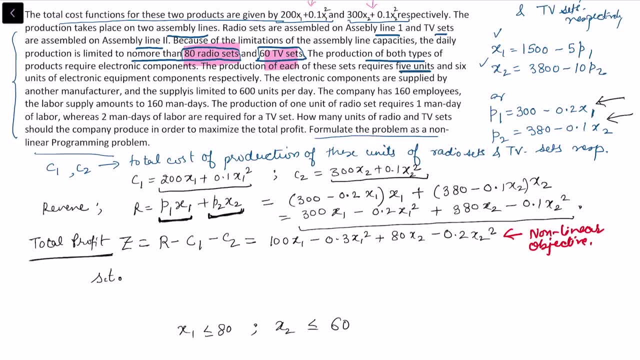 production of each of these sets is less than or equal to 80 and x2 is less than or equal to 60, require five units and six units of electronic equipment component respectively. so that's the another data. we have to keep this in the constraint. five units and six units respectively means first: 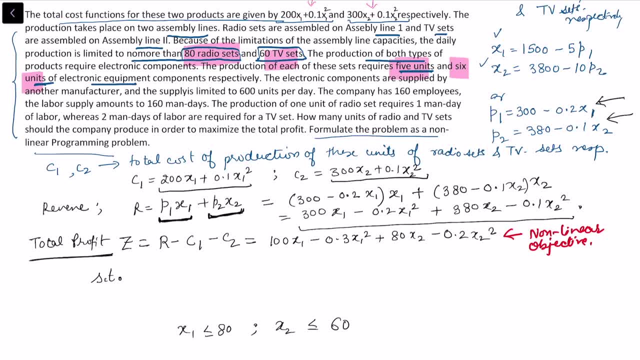 is for radio, second is for tv. the electronic component are supplied by another manufacturer. the supplies is limited to 600 units per day. so this 600 units per day is the capacity of the constraint. so we can simply say: five times x1 plus six times x2 is less than or equal to 600. then there is another constraint: the component. 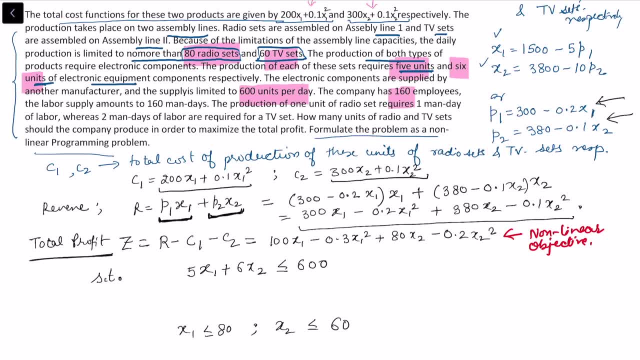 the company has 160 employees and the labor time, labor supply amount to 160 men days. the production of one unit of radius requires one men day and two men day are required for tv sets. so that means for the next constraint we will have x1 plus 2, x2 less than or equal to 160.. so this is the constraint. 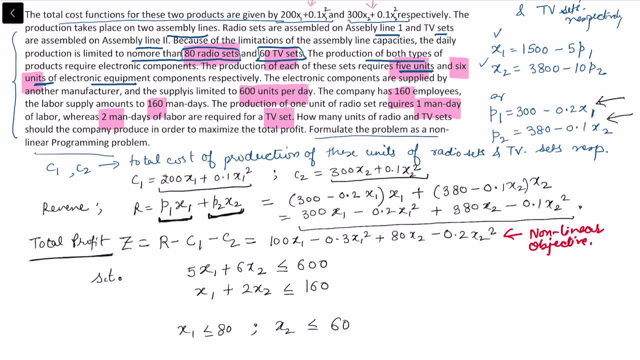 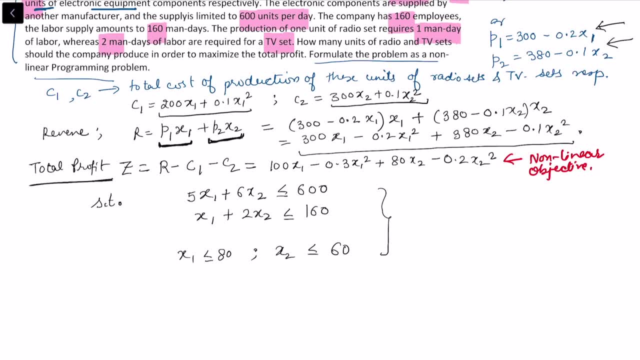 so this is the another constraint. now, looking at these constraints, we can see the constraints are linear, but the objective function is non-linear. so this is the complete formulation and we can also say that this is greater than or equal to zero, because it is a rate, it is a manufacturing. 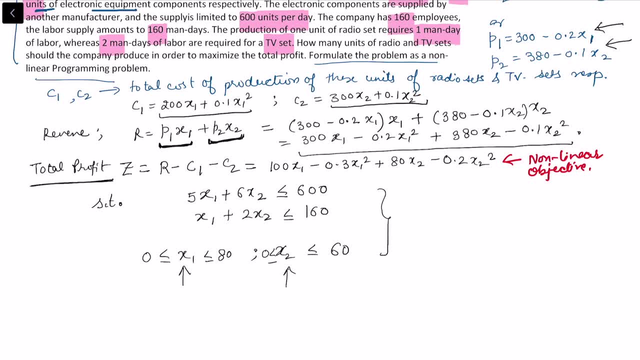 radio and this is the manufacturer tv set, so they cannot be negative. so this is a non-linear programming problem formulation. so we can simply see from this example that if any one of the- either objective function or the constraint- comes as a non-linear, we cannot apply the techniques. 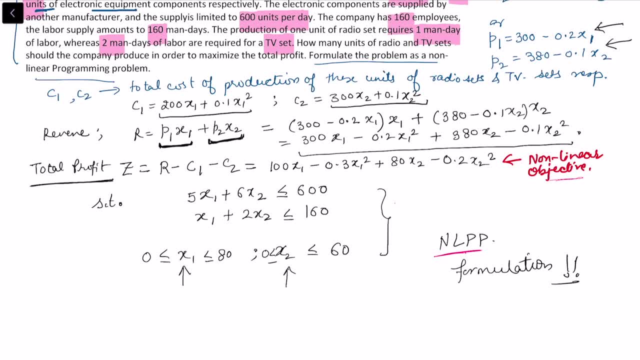 that we have applied for the linear programming problem, but we have to look for the non-linear programming methods to solve these. so i'll explain the methods one by one in my next coming up videos.